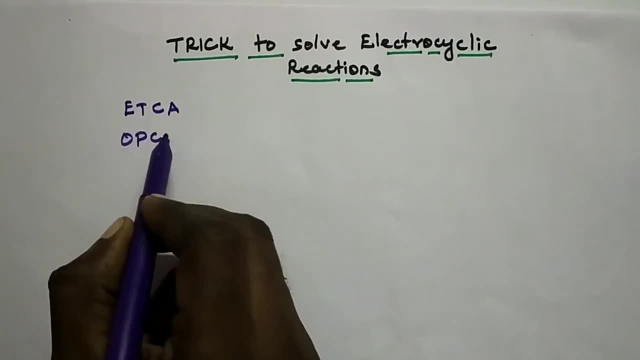 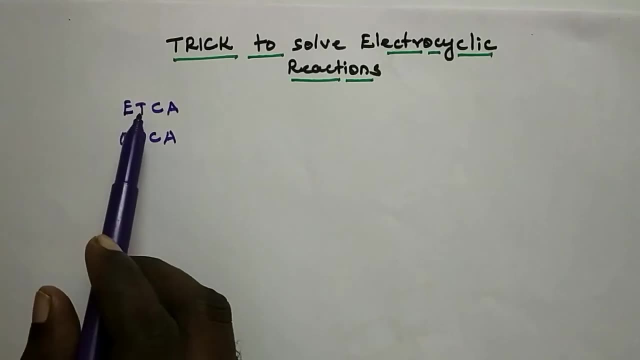 In the previous video. this is what I told you to remember: the Woodward-Hoffman rule. even thermal conrotation anterofacial or photochemical conrotation anterofacial, Since here we are dealing with electrocyclic reaction, this anterosupra is not needed at present. 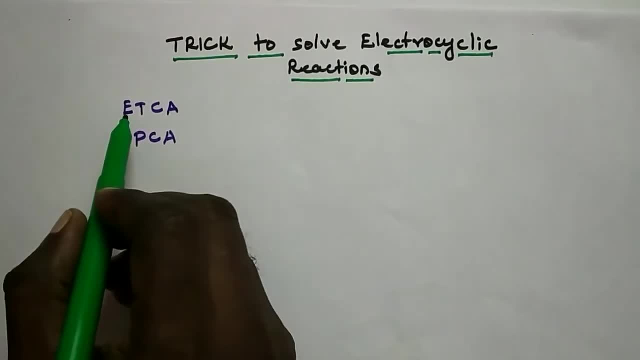 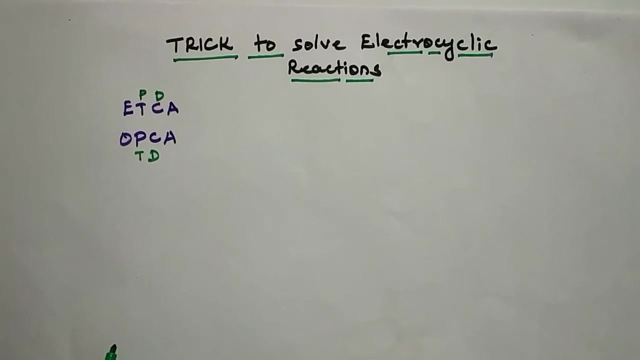 even thermal con or photochemical con. Even Thermal con means photochemical dis, Odd Photochemical con means thermal dis. Okay, Even thermal conrotation, even photochemical disrotation. Odd photochemical conrotation, odd thermal disrotation. This we have already seen. 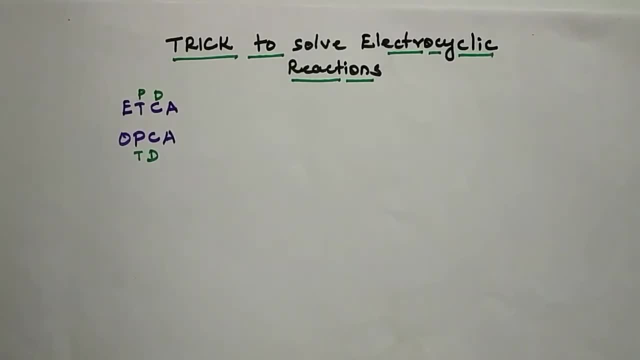 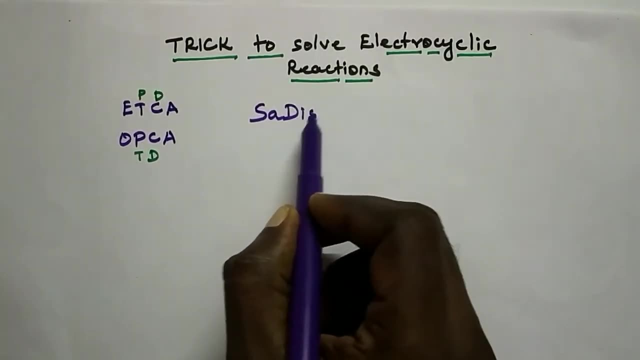 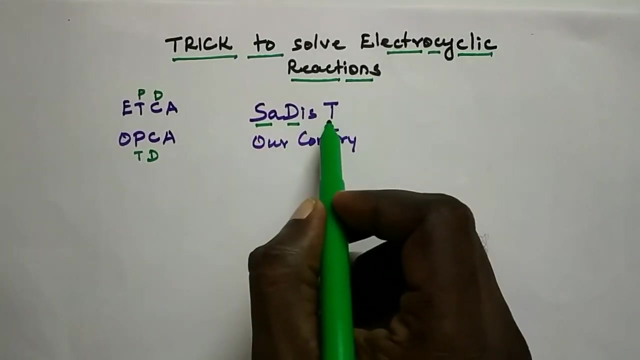 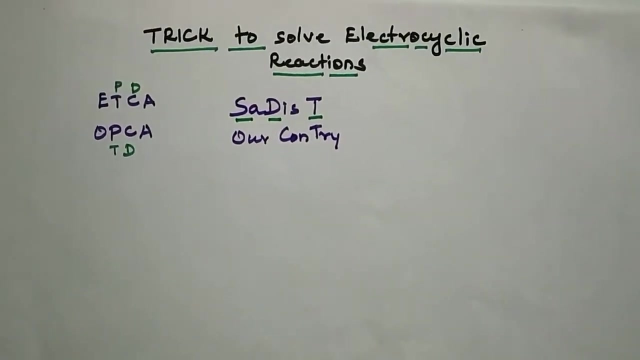 And one more thing I am going to tell you now it is, it is remember this Sadist and our country, our country, sadist, our country. same side- disrotation trans. Opposite side- conrotation trans. 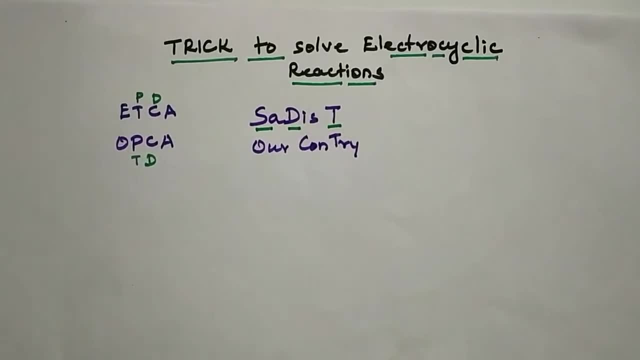 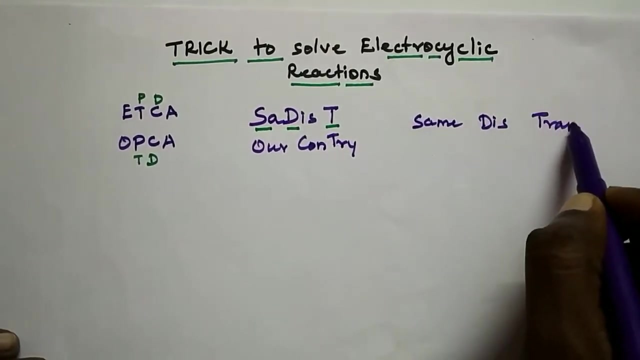 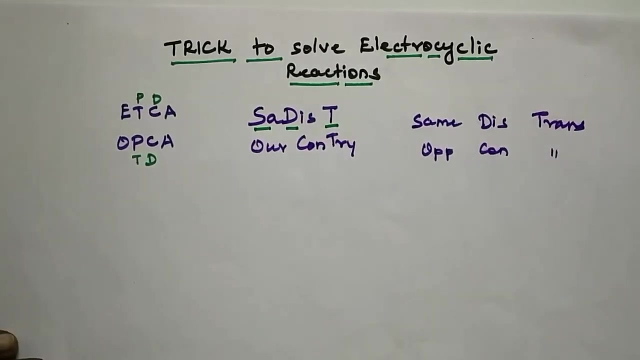 Okay, Yeah, Same side- disrotation trans. Opposite side- conrotation trans. Same side- disrotation trans. Opposite side, conrotation trans. Remember this formula: Okay, Same side, disrotation trans. 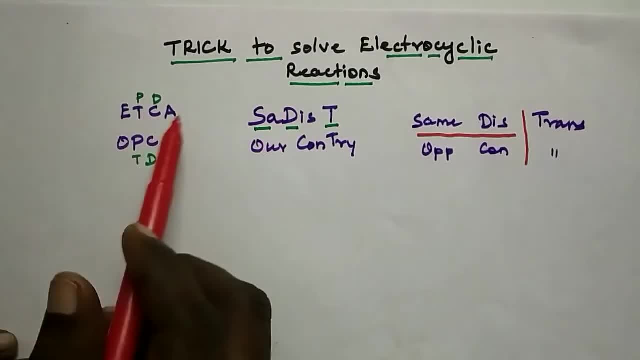 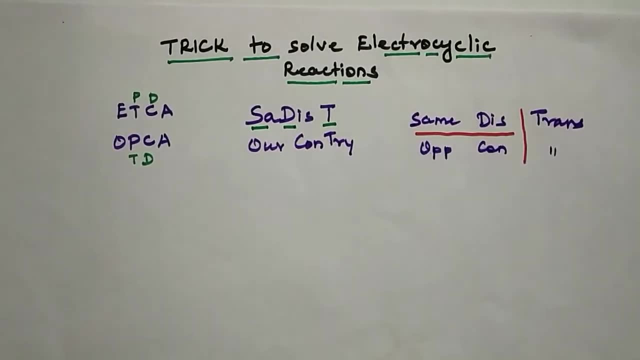 Opposite side conrotation: trans Sadist- our country, Itka oka sadist- our country. This is what you need to remember. This is enough for this entire electrocyclic reaction. Okay, Let us see this reaction. first of all, 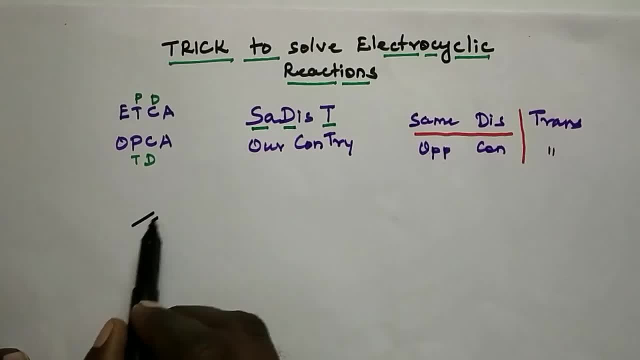 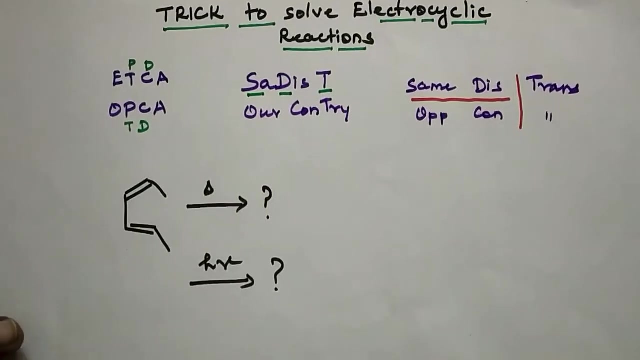 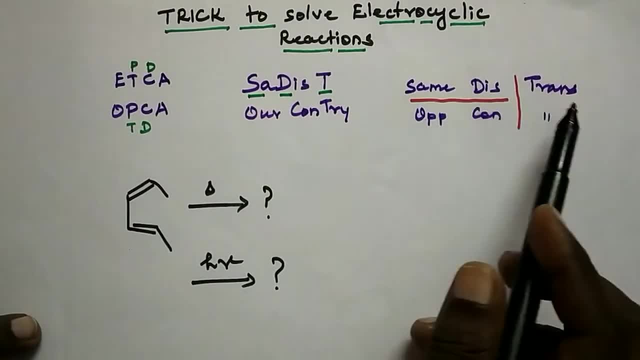 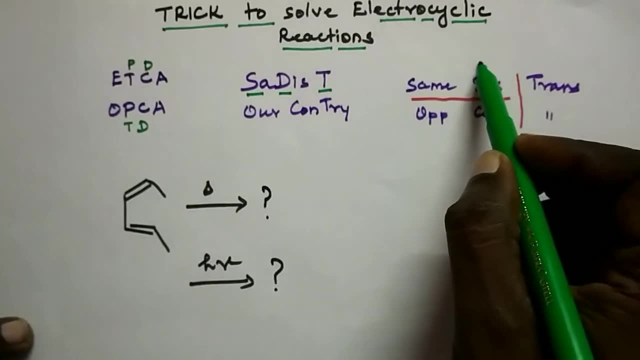 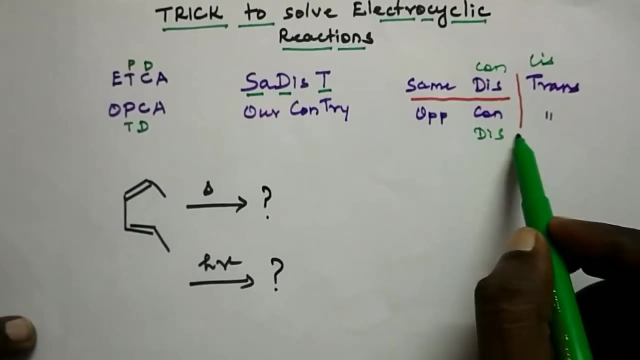 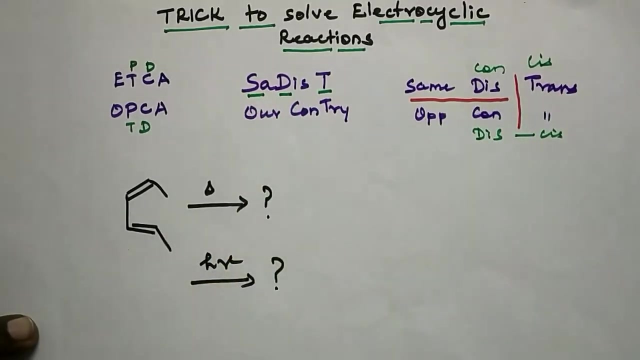 Okay, Okay, Come to this rule. What it says: Same side disrotation trans. Opposite side conrotation trans. Okay, If discon means con will be cis, Contrans means dis will be cis, Cis, isn't it? so you remember the first two? same dis, trance up con trance. saddest our country. 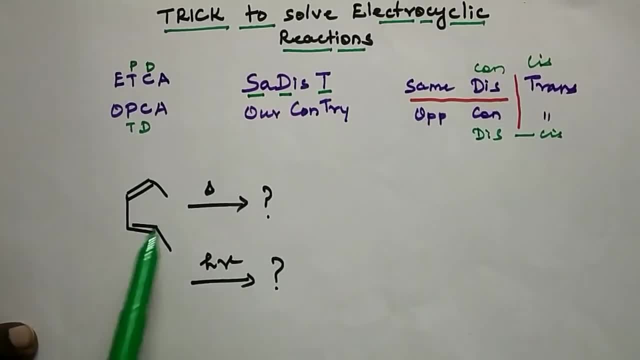 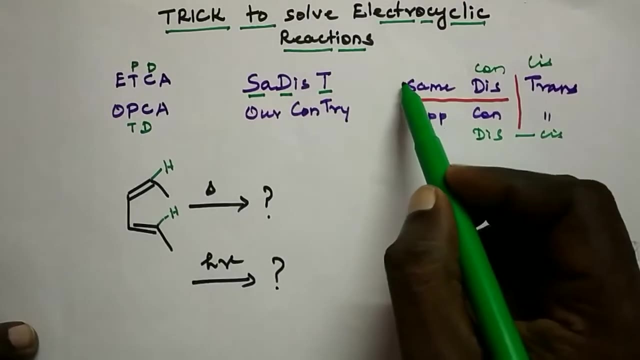 You remember that? okay, now look at that. Now, the products are substitution. look at that. these two are same side, isn't these two? methyl are same side and Hydrogens are same side. So substitution are same side, Substitutions are same, right here. Okay, same side, same side. 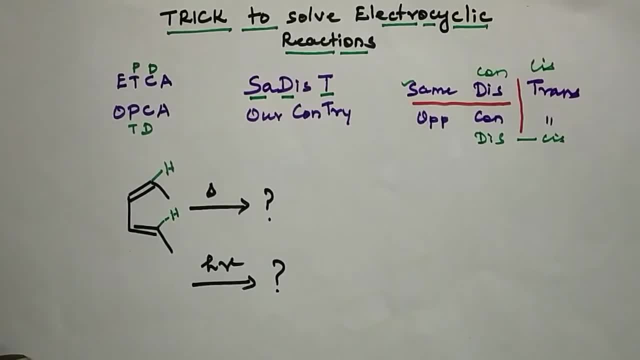 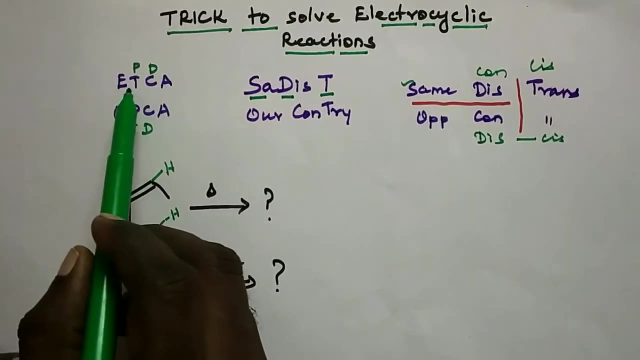 This rotation trance con rotations is whether it is this at con. How can you find out? look at this. this is thermal condition. What is the rule? says: even number of pi bonds to pi bonds, even number, even thermal con etka, oka Etka, even thermal con rotation here: even number, thermal condition. so it is con rotation. 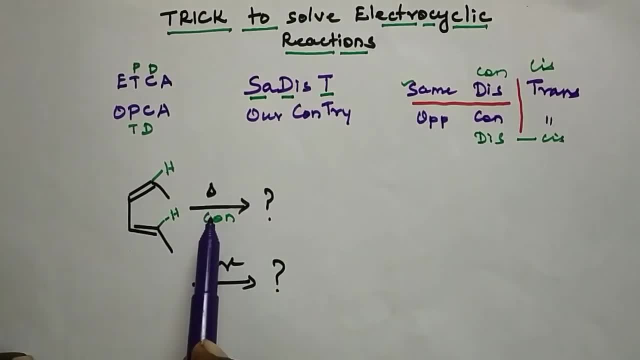 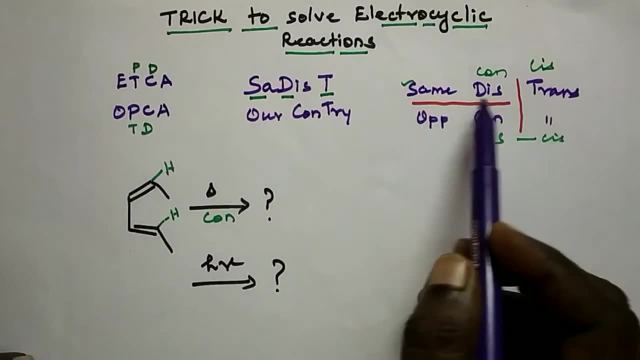 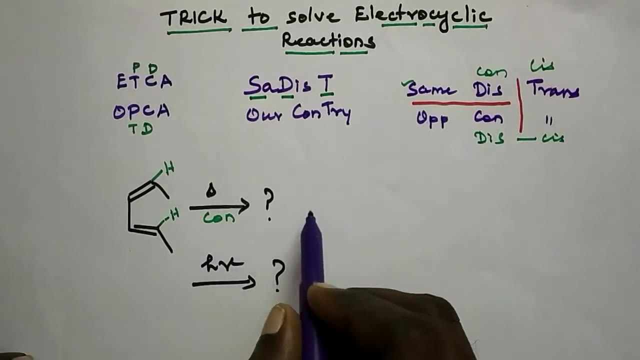 Okay, now rotation is con. Rotation is con. substitute: one: same side, okay, Same side, con. look at this: saddest, Saddest: same side: dis rotation trance, so same side, con. rotation is cis, so the product is cis product. So we need to. The product is like this: cis product, okay, cis product. 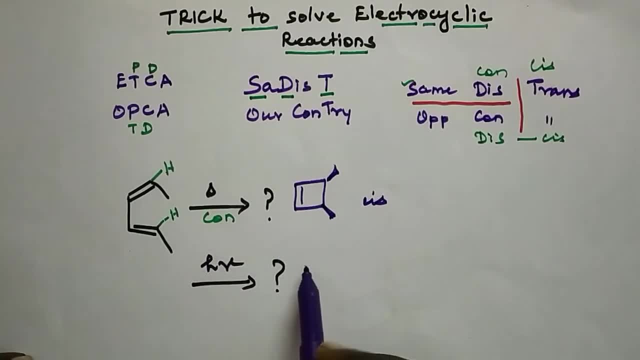 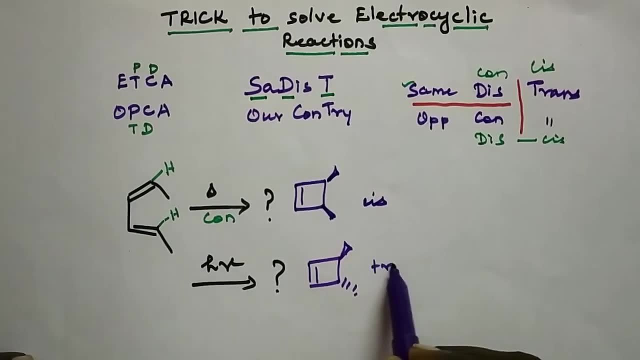 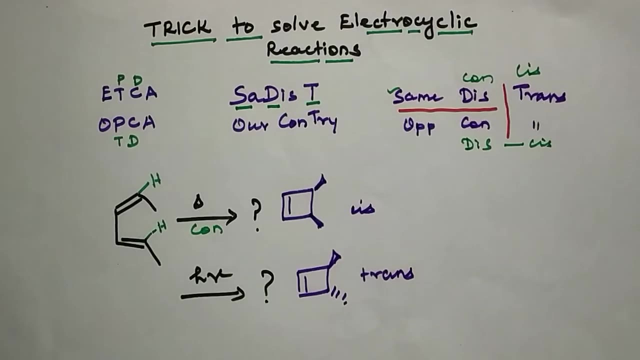 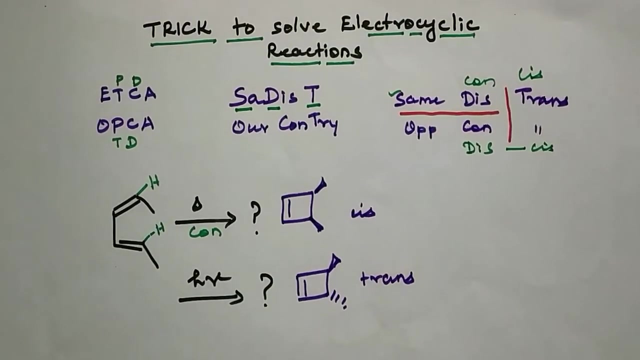 Okay, thermal condition, cis means photochemical condition. obviously it is trans product, Trans. Hope you understand. remember etka oka, Etka oka. and remember saddest and arcant, same side, this rotation trance, opposite side, con rotation Trans, saddest arcant. remember that and let us see these problems. 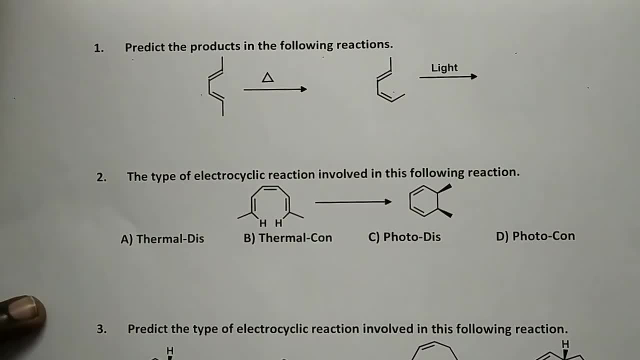 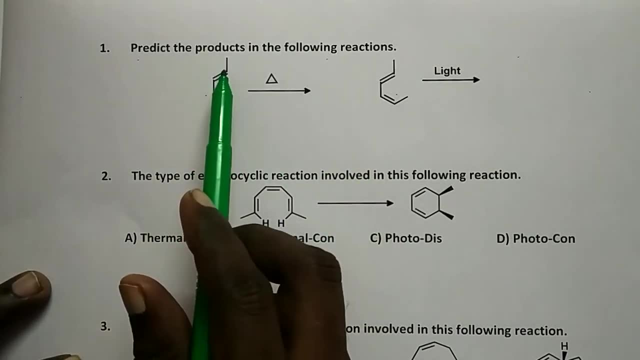 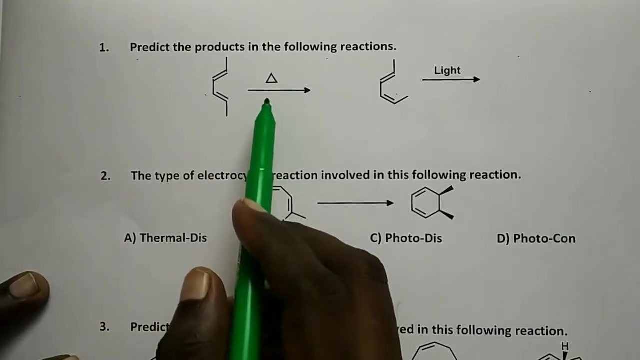 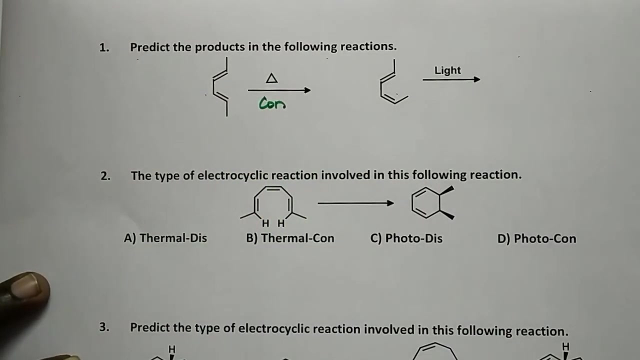 you see, predict the Product and the following reactions. Look at this Opposite side, isn't it opposite side, okay. thermal condition, Thermal condition. first find out whether this is that trance. Even number of pi bonds con rotation etka. even thermal con con rotation. thermal condition con rotation etka. okay now. 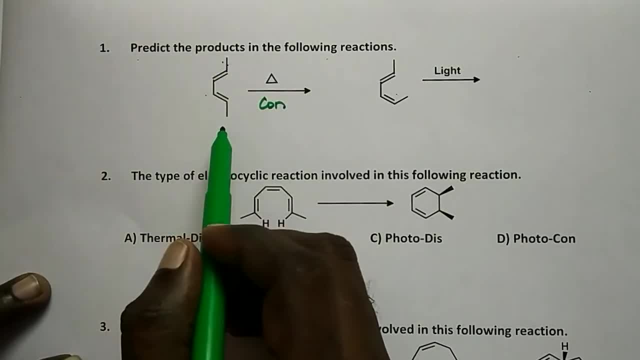 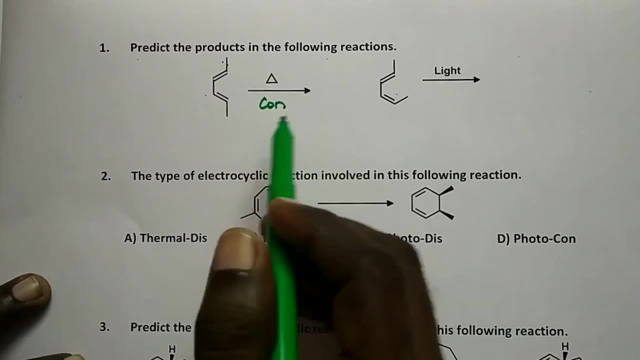 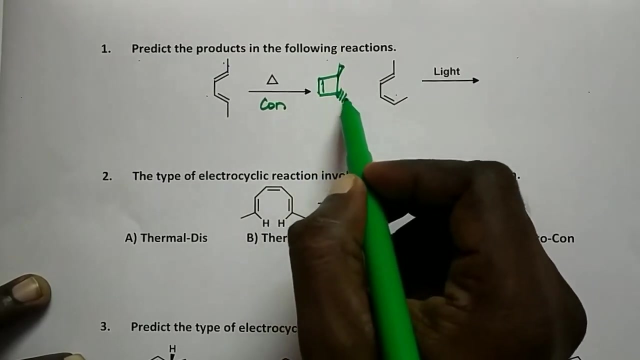 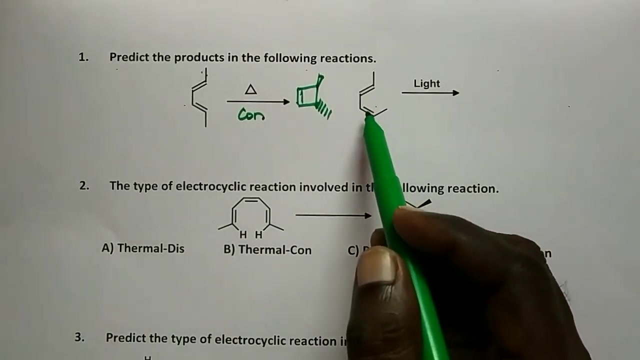 Substituent. opposite side, opposite are same opposite side, Opposite side, con rotation. What is it? our country, Opposite side, con rotation, trance. so the product is trance product. Okay, product is trance Trans product. and look at this one Here also two pi bonds, even number. 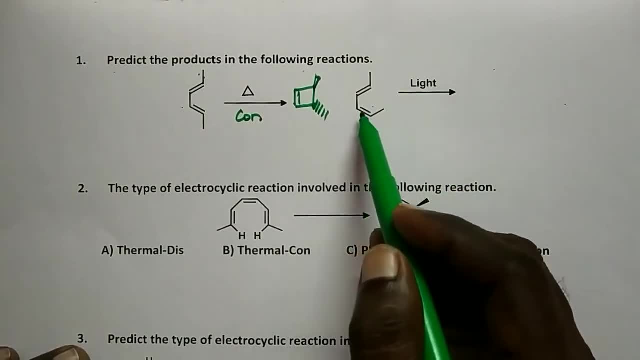 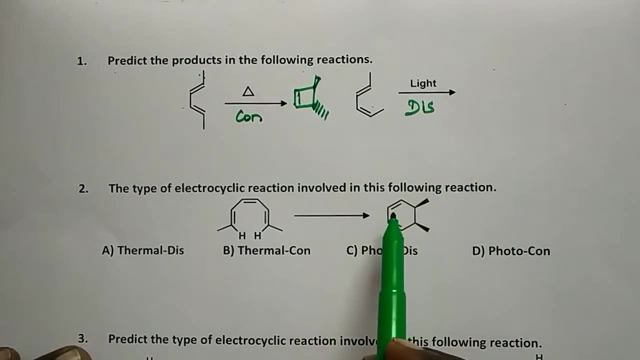 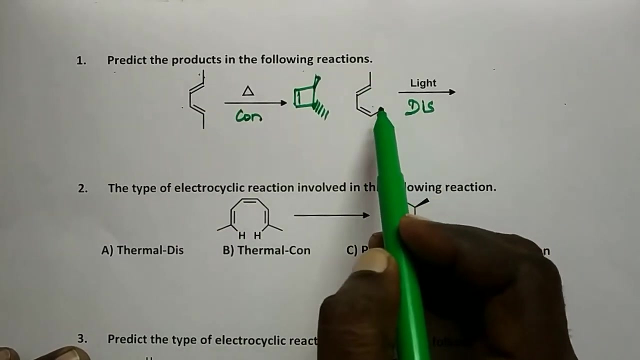 photochemical condition, okay, even thermal con means even photo, this rotation, etka oka. even thermal con, even photo this. Now look at the substitutions, substitutions, same said here It is opposite side, here same side, Same side. this rotation saddest, saddest means trance, okay. 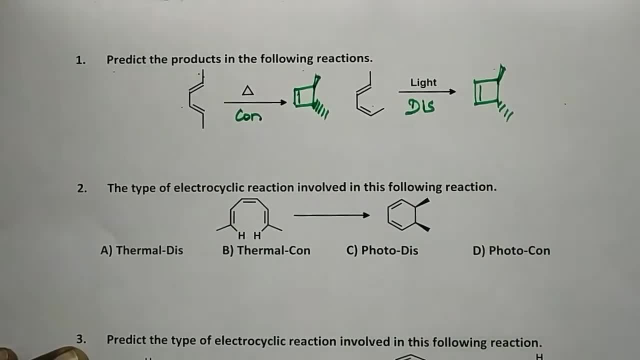 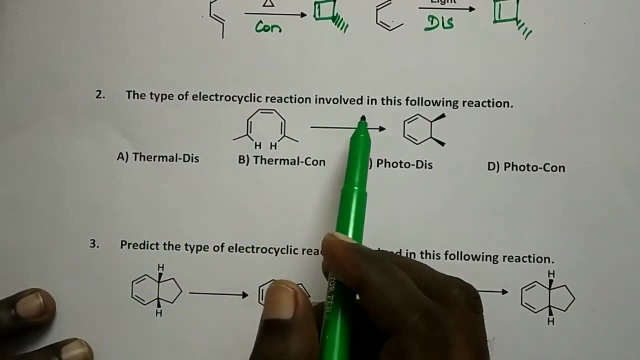 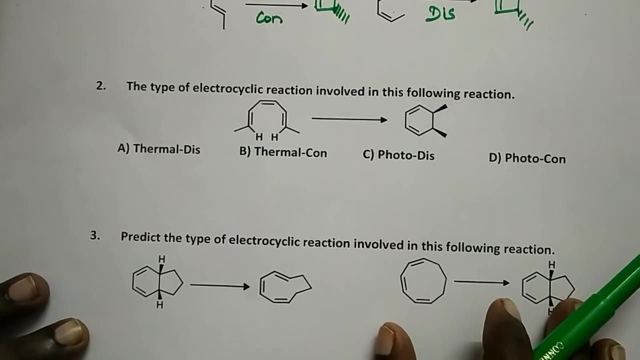 So product is a trance product, trance product. Okay, let's go to the next one: the type of electrocyclic reactions Involved in the following reaction. what sort of electrocyclic thermal? this thermal con photo, this photo con. okay, What is it? 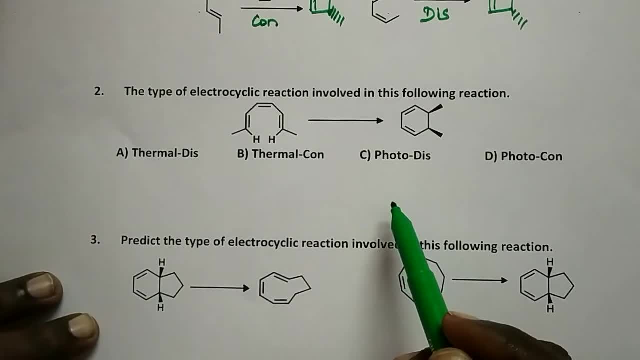 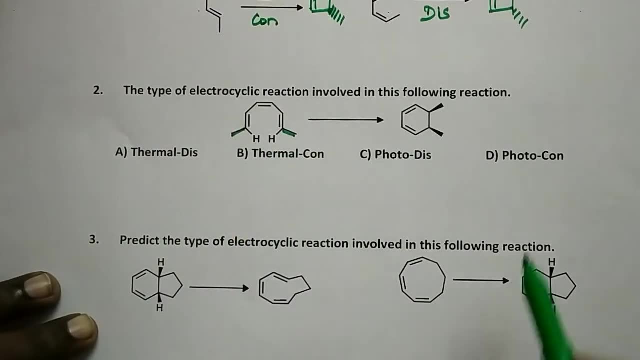 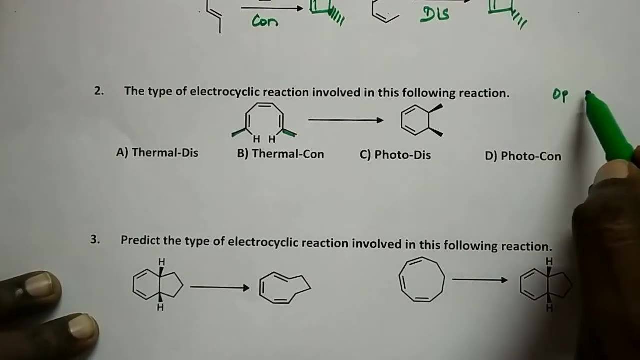 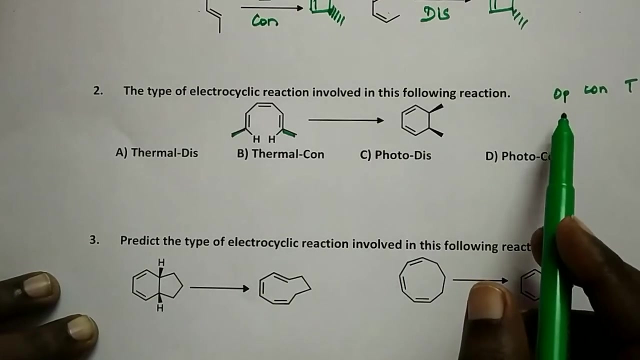 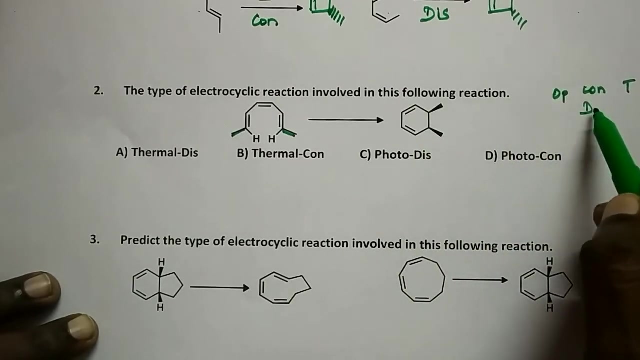 Look at the product. it is this sis product. Okay, look at the substitutions of the starting material: same side or opposite side, opposite side, opposite side. this rotation, What is that? our country, our country, opposite side, con rotation, trance, trance. Opposite side, con rotation, trance. Here we get: product is sis, so it should be what this rotation? the rotation is this. that is why sis product. 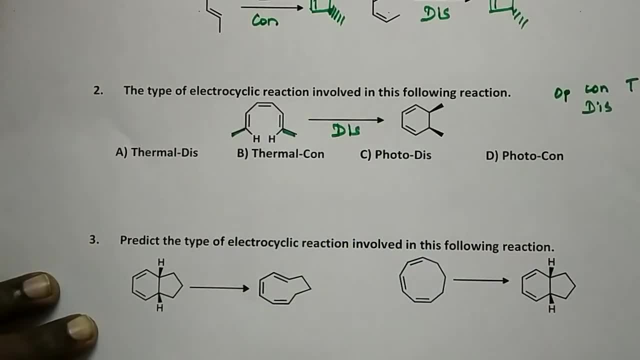 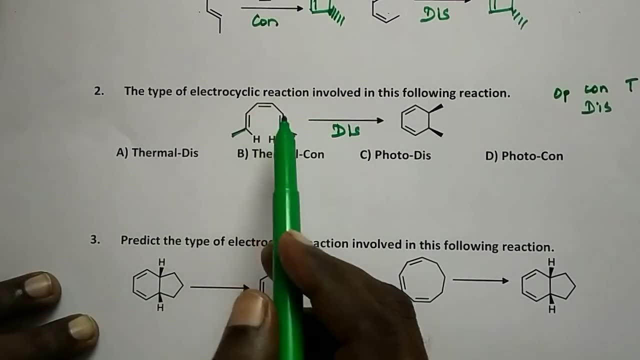 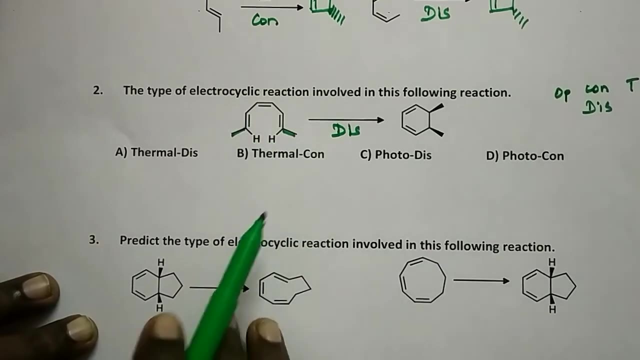 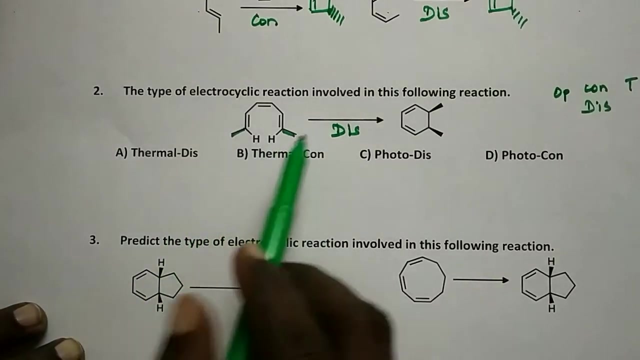 So rotation is this rotation? Okay, rotation is distraught. means whether it is thermal or photochemical. look at this: three pi bonds odd number: etka oka odd. thermal. etka oka odd. Sorry, yeah, etka oka odd. photochemical con rotation. Photochemical con rotation means: here we have this rotation, so it should be. 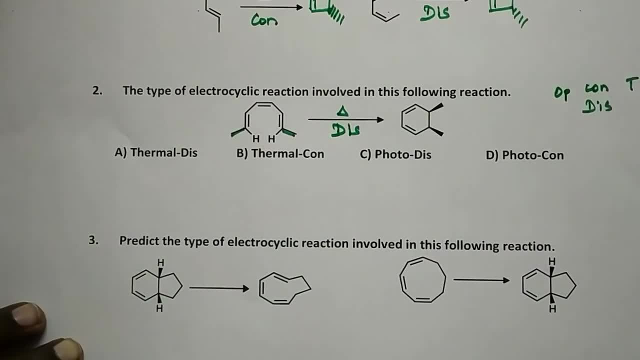 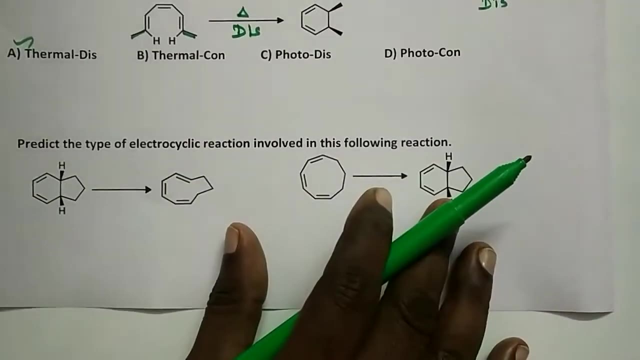 thermal okay. Oka photo: chemical con rotation. since we have this rotation, Conditions would be thermal okay. so, thermal, this rotation, thermal this rotatory ring closure- Ring closure: okay. and let's come to this one. Look at this: Predict the types of electrocyclic reactions involved in this following reactions: 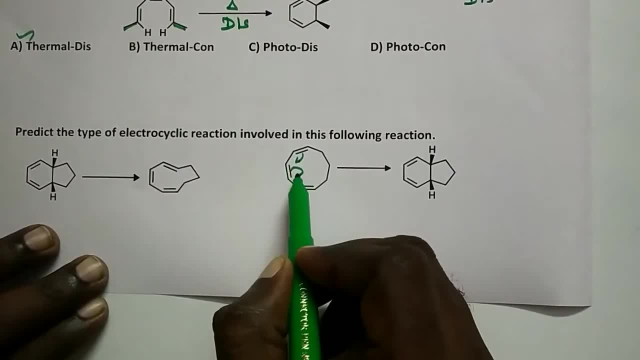 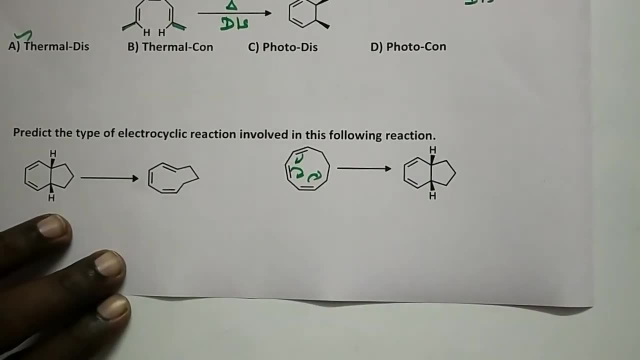 Let's see this one first. This is a ring closure, electrocyclic ring closure. Product is sis product Substitute one same side or opposite side Substitutes. look at the hydrogens: hydrogen hydrogen. so Substitutes are opposite side. okay, Opposite side. 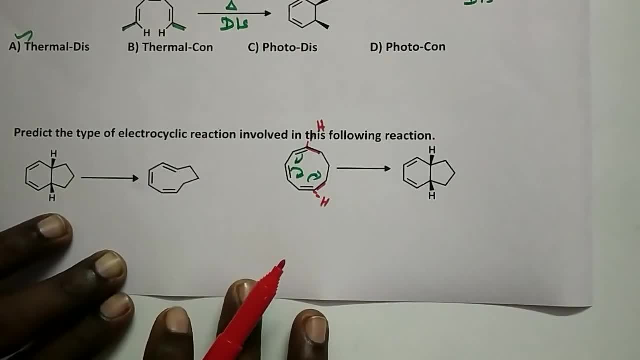 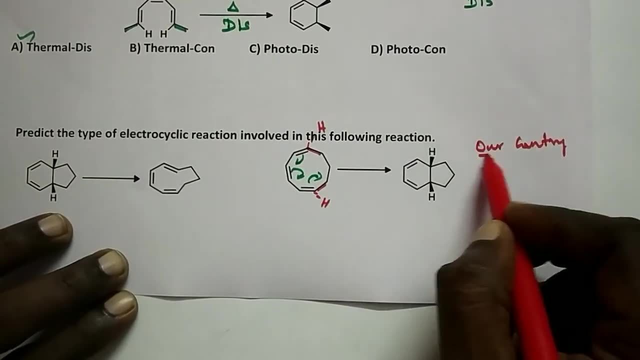 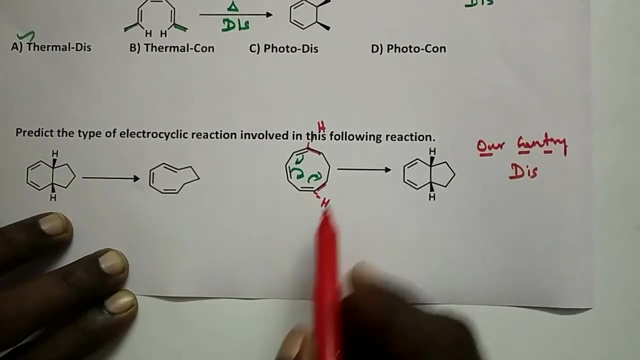 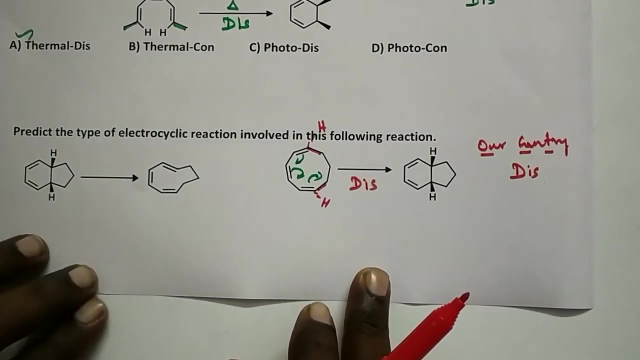 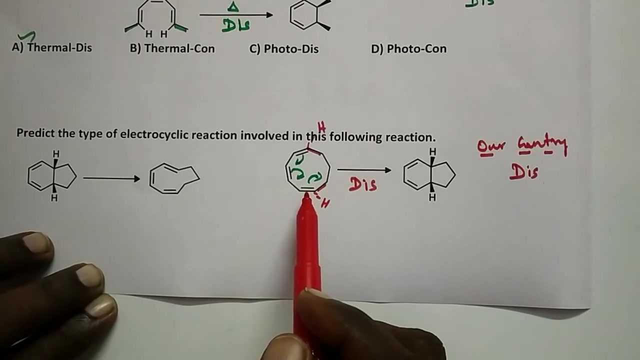 Opposite side, sis. what is that? our country, our country, our country, Opposite con trans. but here we have sis product. so it should be what? this rotation, this rotation, okay, Odde, Odde, con rotation, trans. so this rotation, sis, This rotation is this Now see, thermal or photochemical. When will you get this rotation? 1,, 2,, 3,, 3 pi bonds, odd number, Oka, odd, photochemical con rotation. So this means it should be thermal. 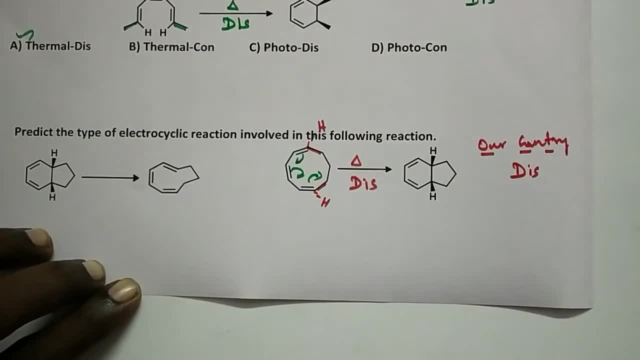 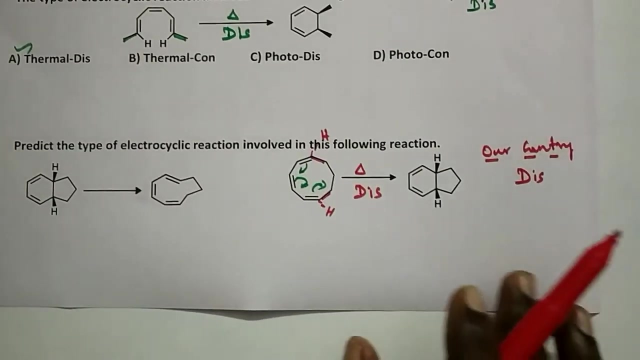 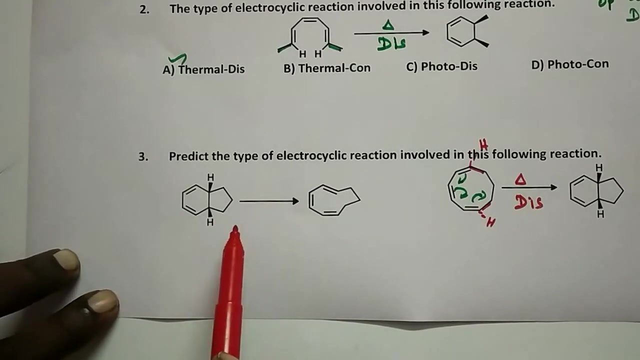 Oka, odd photochemical con rotation, But since the rotation is this, it should be thermal condition. So thermal dis-rotatory ring closure. electrocyclic ring closure. Come to this one, And this is different. This is a new thing. We have never discussed about this earlier. So here ring closure, it is not ring closure, Here, it is ring. Oka, odd photochemical con rotation, But since the rotation is this, it should be thermal. So thermal. dis-rotatory ring closure. Electrocyclic ring closure. Come to this one, And this is different. This is a new thing. We have never discussed about this earlier. So here ring closure. it is not ring closure, Here, it is ring. 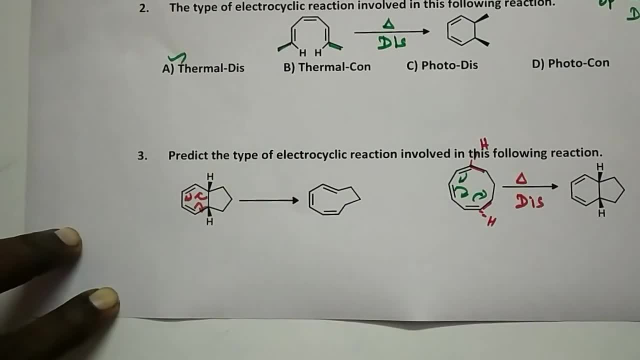 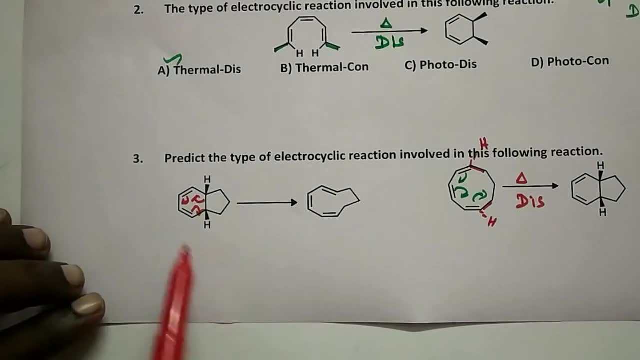 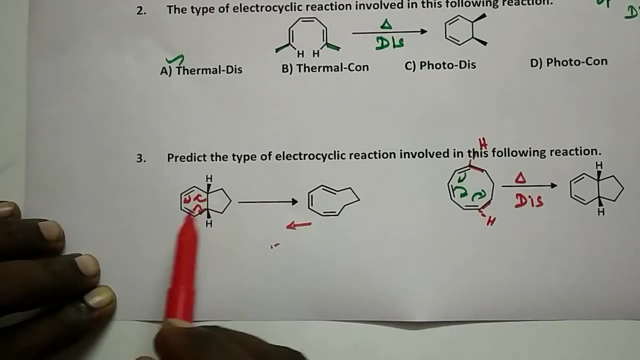 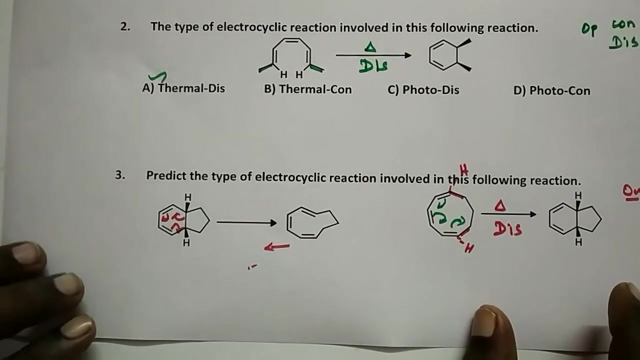 Oka, odd photochemical con rotation. But since the rotation is this, it should be thermal, So this is different. This is a new thing. We have never discussed about this earlier. So here ring closure. it is not ring closure. Here it is ring. 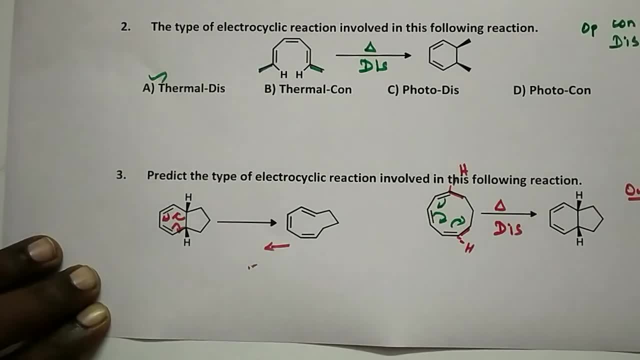 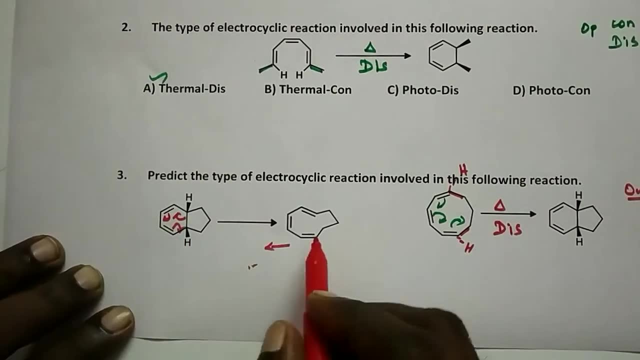 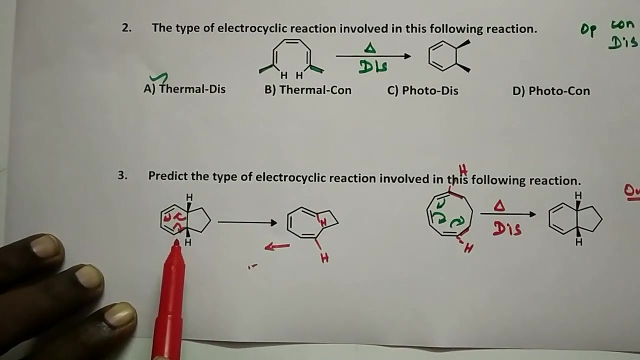 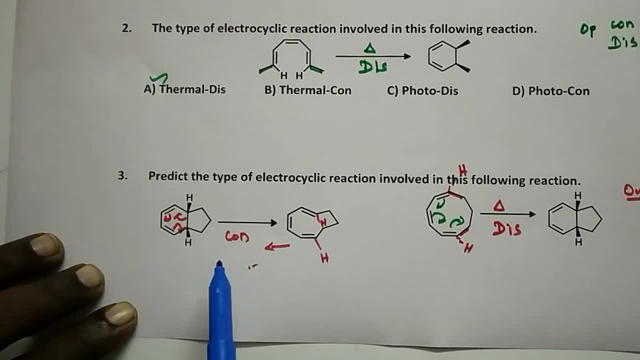 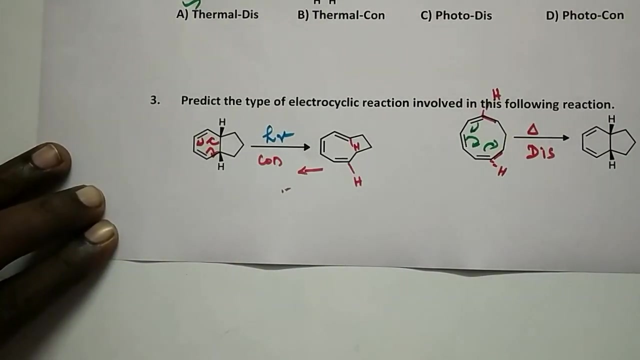 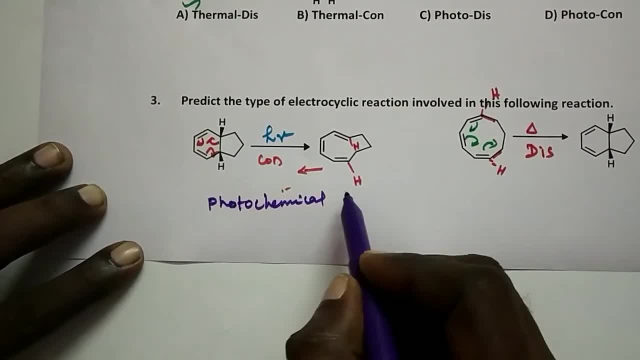 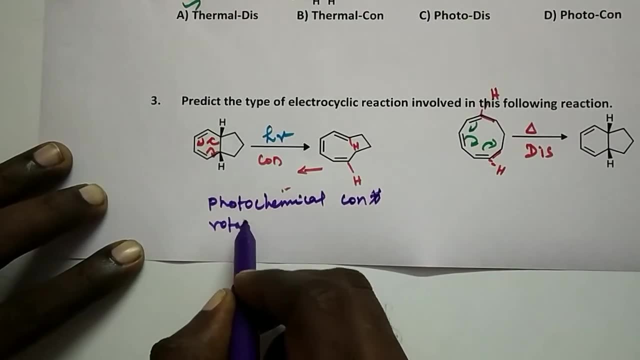 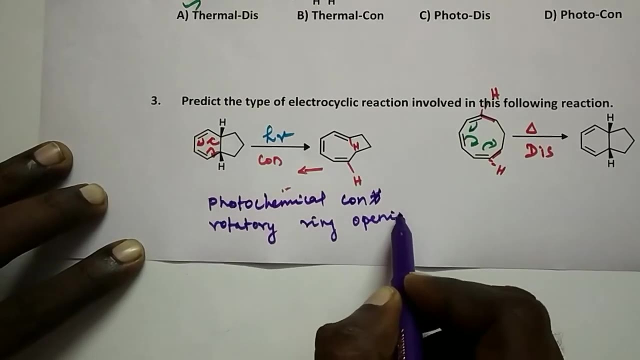 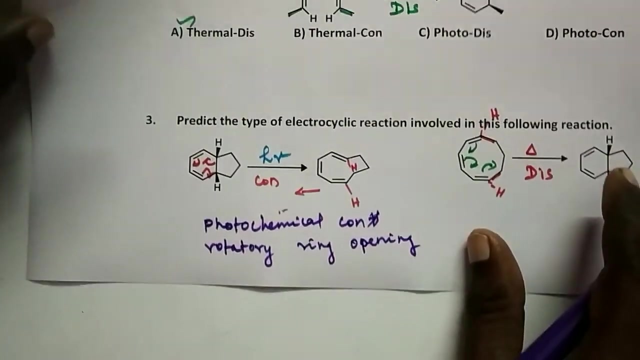 Photochemical conrotatory, conrotatory, rotatory ring opening. These are all ring closure. These are all ring closure, But this is ring opening. So we need to say photochemical conrotatory, electrocyclic ring opening. 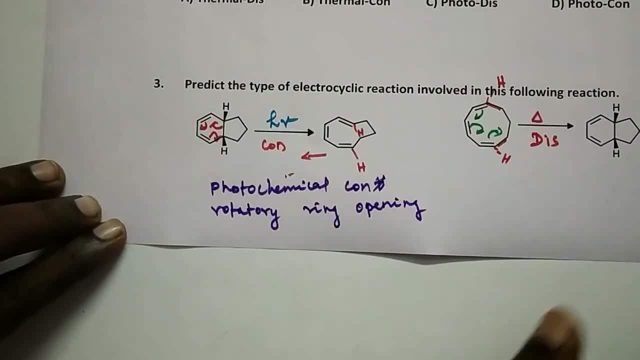 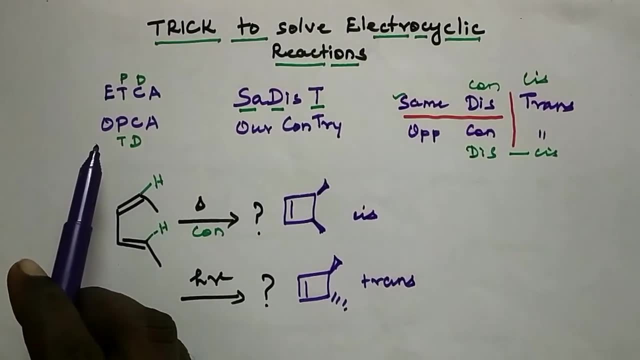 Again: photochemical conrotatory, electrocyclic ring opening. Hope you understood The two formula you need to remember. This is what, once again, I tell you: etka, opka. We have already seen that: Etka opka. 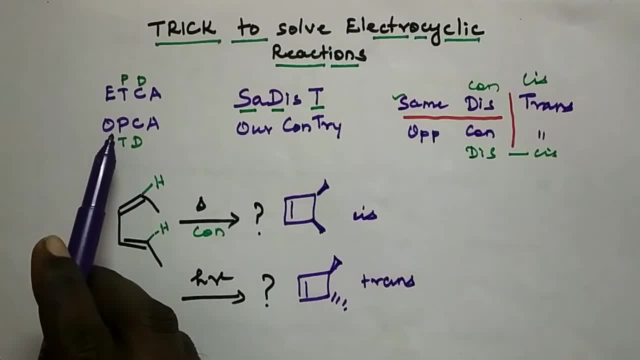 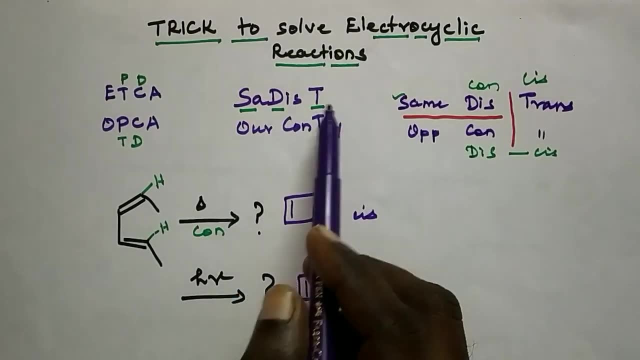 Even thermal conrotation anteroficial, Odd, photochemical conrotation anteroficial, Etka, opka. And one more thing is saddest: arcantry. Same side, disrotation trans. Opposite side, conrotation trans.